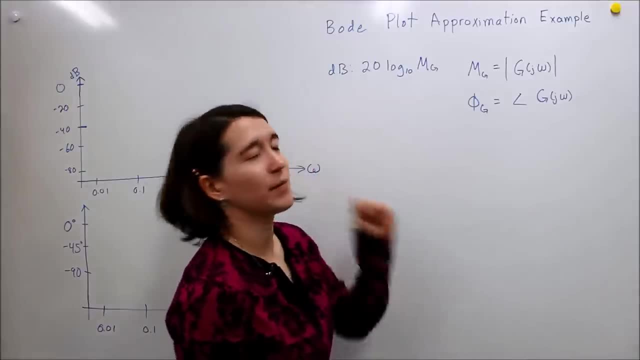 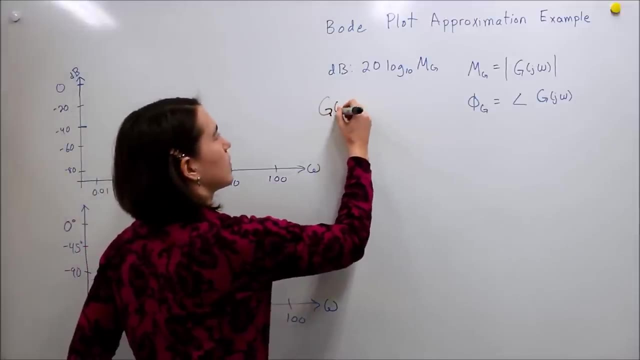 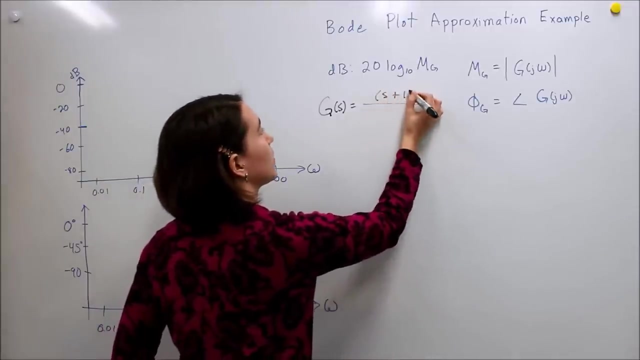 We're going to work one more problem using the Bode plot approximation for the frequency response And we're going to look at a system that has one zero and two poles. So if we have a system of one pole s plus one, sorry, zero. 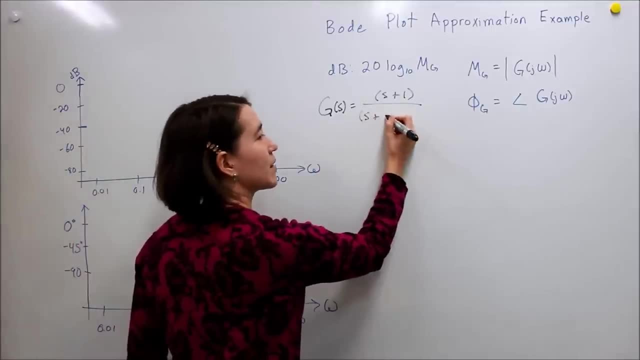 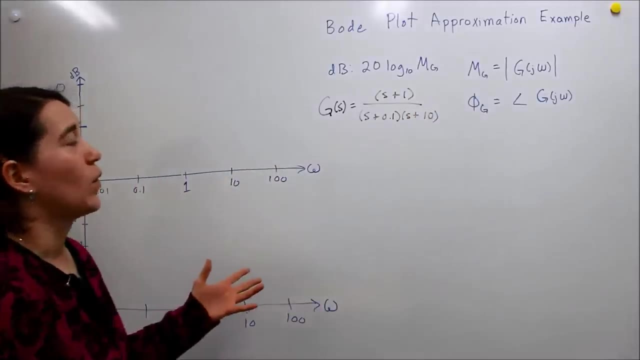 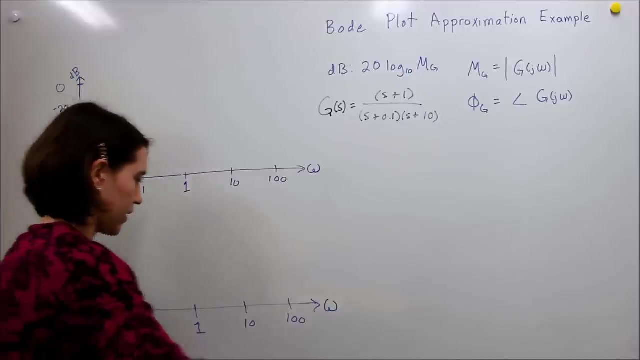 Zero at negative one, and then we have s plus 0.1 and s plus 10.. So we have two poles. What does this look like if we take the frequency response of it? Okay, so we are going to do the way I like to start. a problem is to look at first what the system looks like at very small values of s. 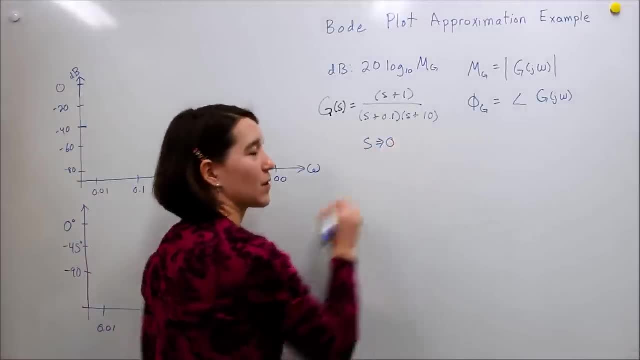 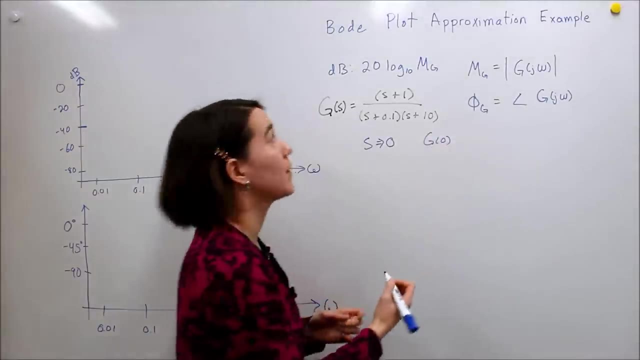 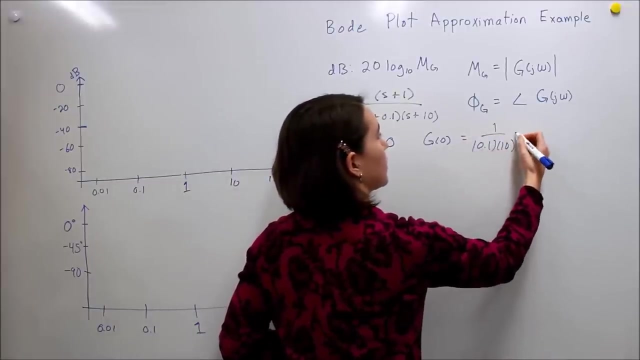 So if s equals zero or approaches, I guess it goes towards zero. In this case, we see that if we take g of s, s equals zero, we're going to get just one Divided by 0.1 times 10, which is just equal to one. 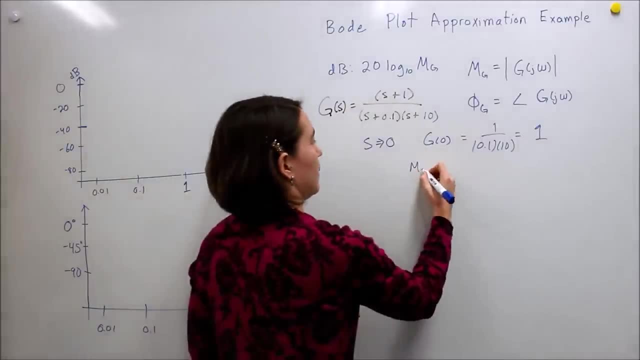 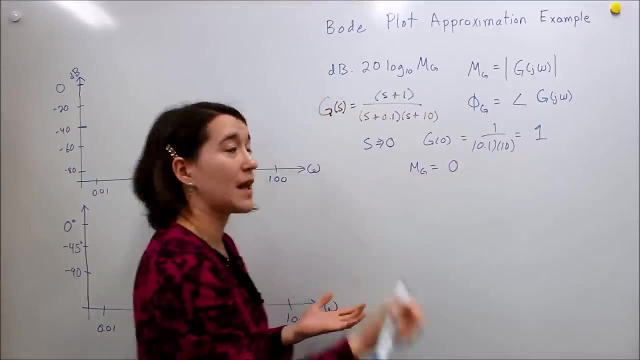 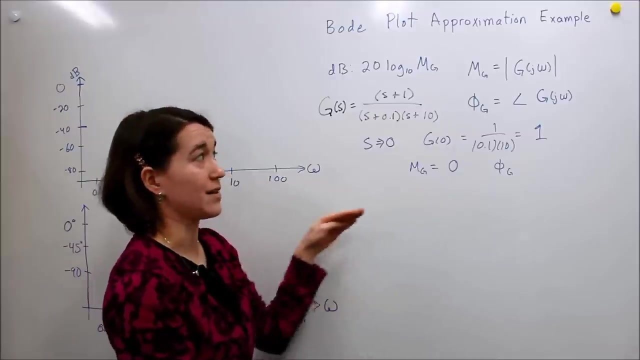 So if we take the magnitude of that, that's going to be: log 10 of one is zero, so we have zero. And if we look at the angle of that, so phi of g here is going to be: well, one is positive on the real axis, so we're going to have zero degrees. 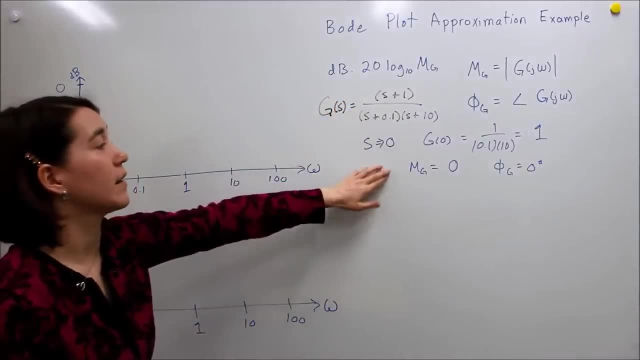 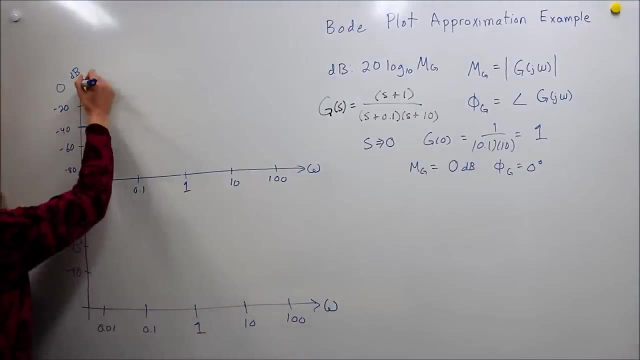 So at very small values. we know that this system is going to look like this. It's going to look like a zero. this is zero dB and zero degrees. So we can start by just drawing that out here. So here we have: zero dB. we start here. 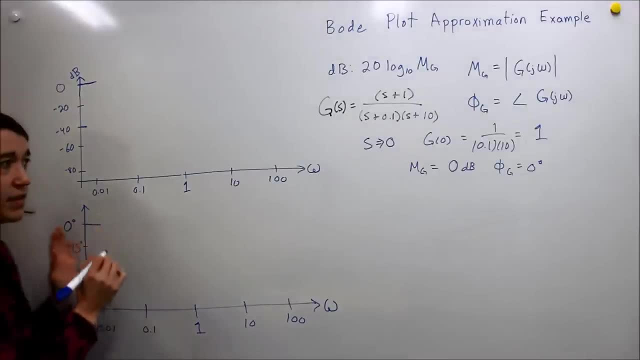 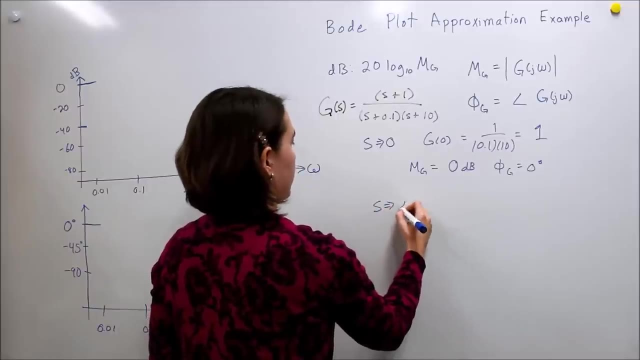 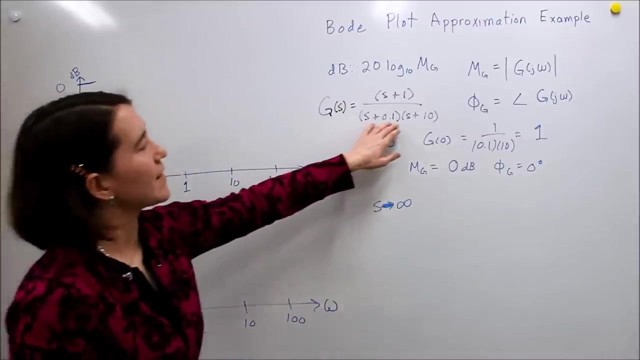 Here we have zero degrees. we start here, Okay, And then at the end, as s goes to infinity. I guess there should just be one line there, As this goes to infinity. what does it look like? Well, as s gets very large. 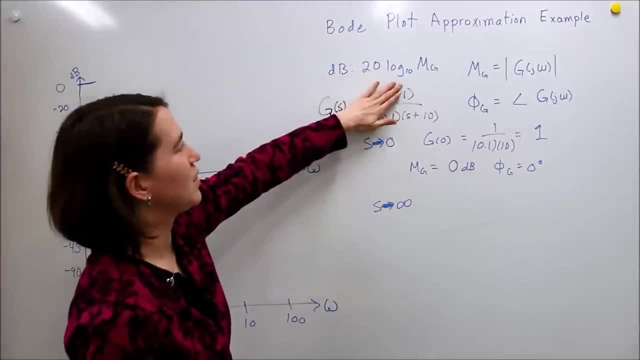 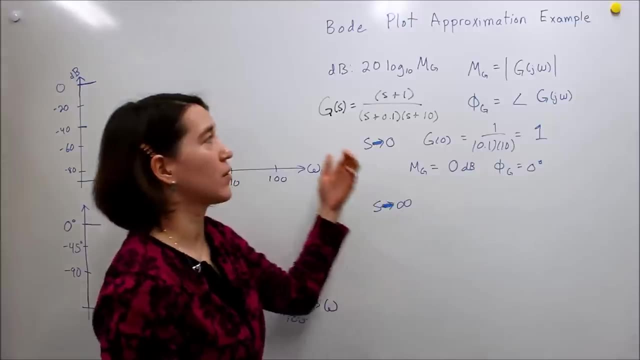 the s's are the only thing that matter. So we'll have these two will effectively cancel each other out. one zero and one pole, and we'll have just one pole left, So it'll look like one over s If we look at the magnitude of that. 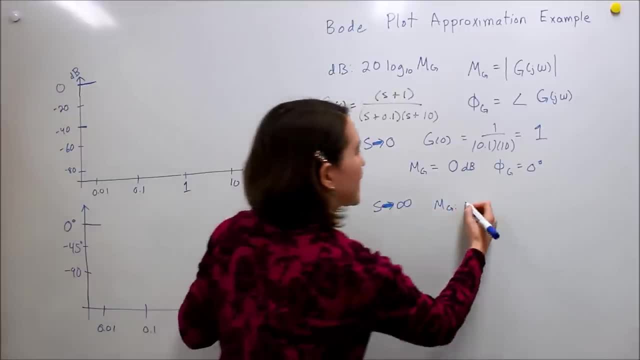 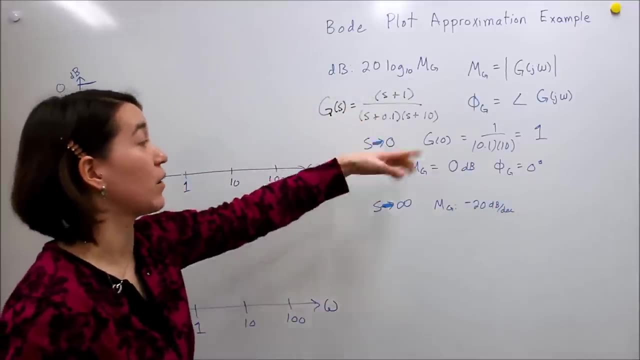 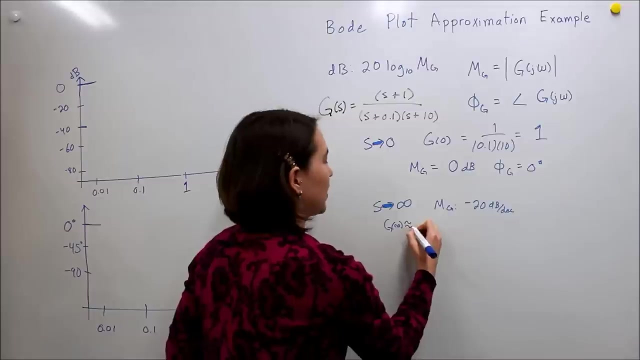 well, we don't know the exact value, but we know that it's actually decreasing at 20 dB per decade. And then, if we look at the angle, we do know the angle of one over s, So g of of infinity, approximately will look like one over s right. 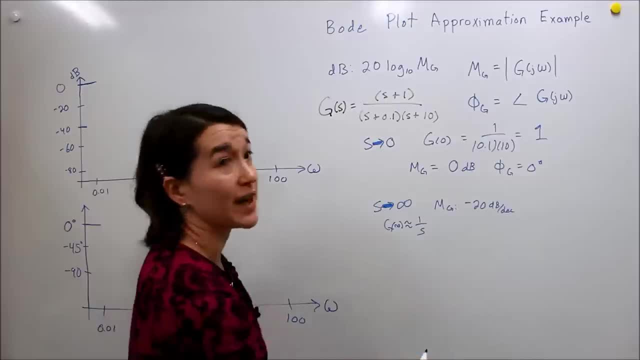 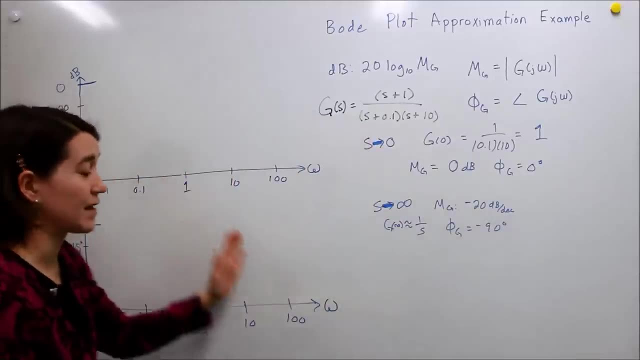 And so we know the angle of that is going to be negative 90. So g is equal to negative 90 degrees here. So that's as we go to infinity. So we don't know exactly what will happen. We'll know we'll end up about at 90.. 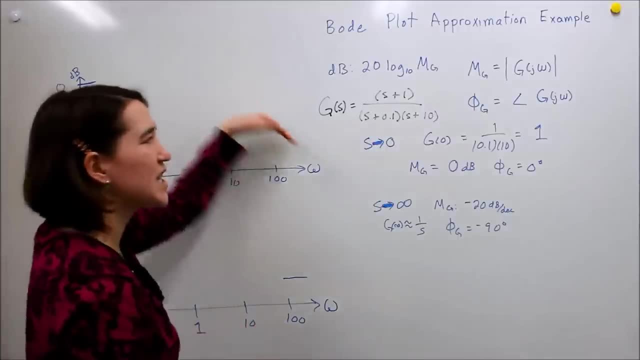 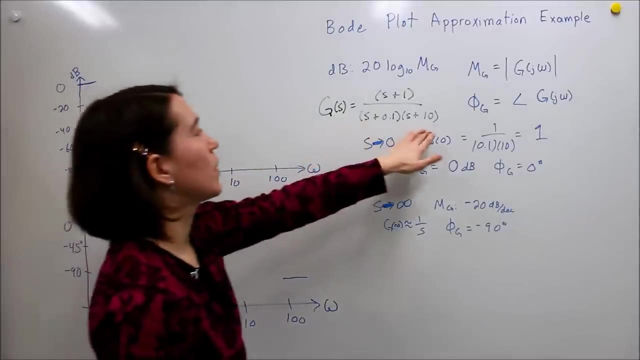 Let's see my graph here from 90.. And we'll be decreasing. We don't know exactly where yet, so I won't draw the line here. Okay, So now let's look at what happens as we go through where these poles are located. 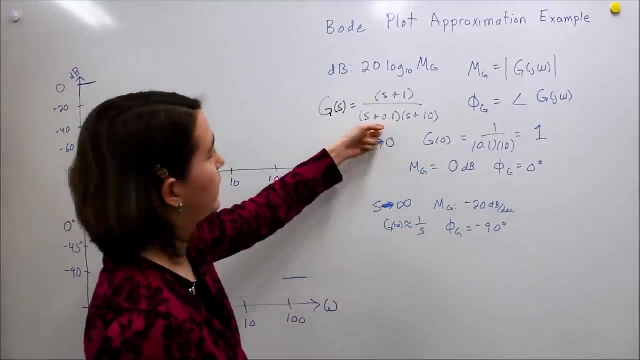 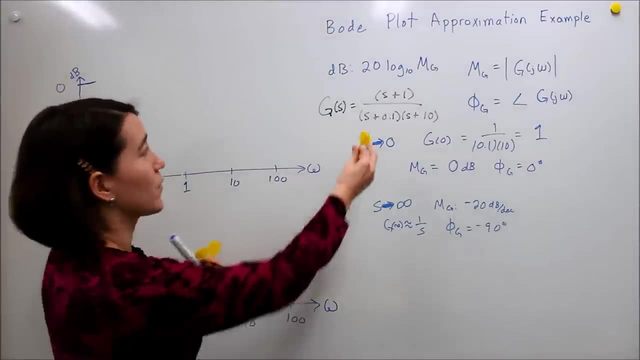 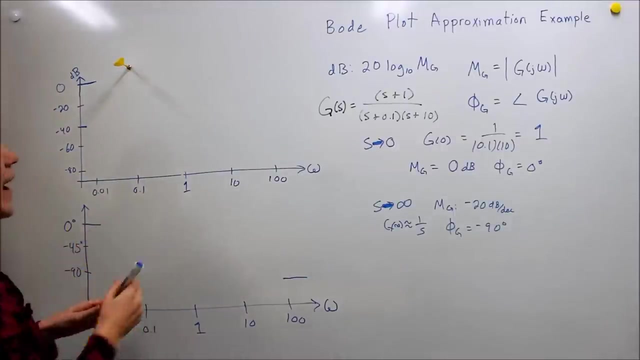 So the first one, the lowest value one, is 0.1.. So I'm going to try to use some creative darts here. So the first one is 0.1.. So we have pole effect here And that will start changing the magnitude. 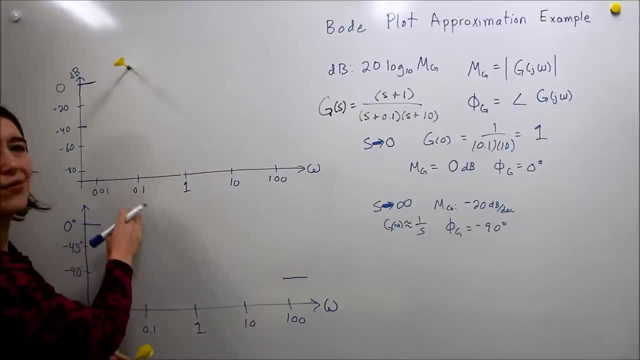 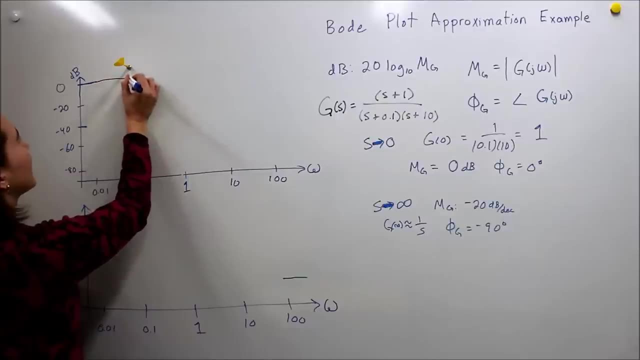 once the magnitude crosses that threshold of this value. Now this is the approximation right. So we know it will start to affect it before we get to this point, but we approximate it as a straight line until then. Once it hits this point right, this first pole, 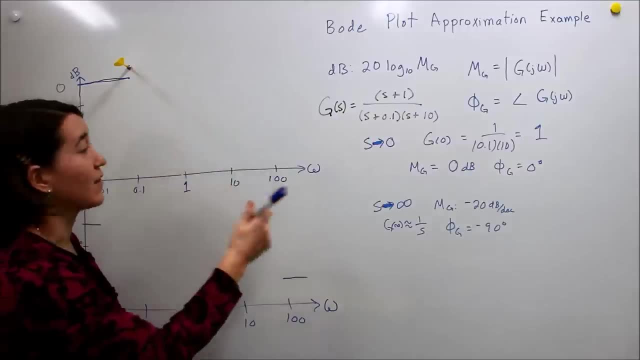 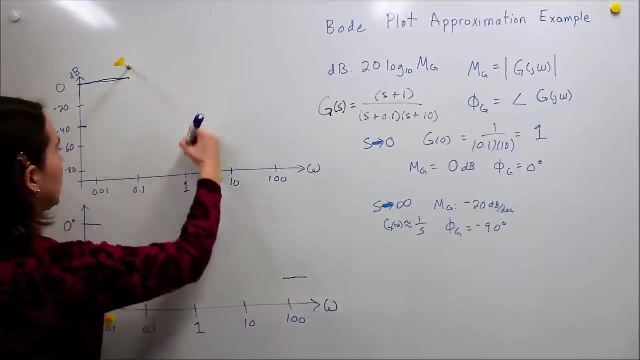 it'll start to decrease at negative 20 dB per decade, because that's the effect of the single pole. So it'll decrease at 20 dB per decade. So here's our next decade: Negative 20.. Go to this point, Okay. 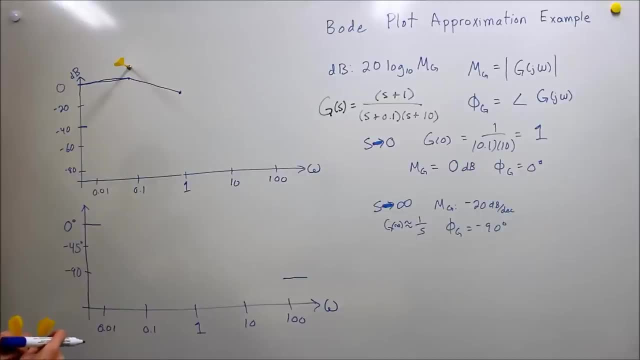 And the effect of the phase is plus or minus one decade. So the effect of this one pole is actually going to affect the phase from 0.1 to 1. And it will affect the phase by making it try to decrease by negative 45 degrees per decade. 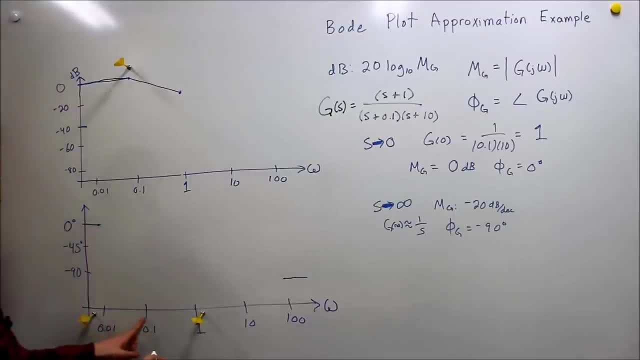 So we can start drawing that one. So we'll draw up to here. So we are going to see it decrease by negative 45. It decreased by negative 45 degrees per decade, So we'll get approximately to 45 right here per decade. 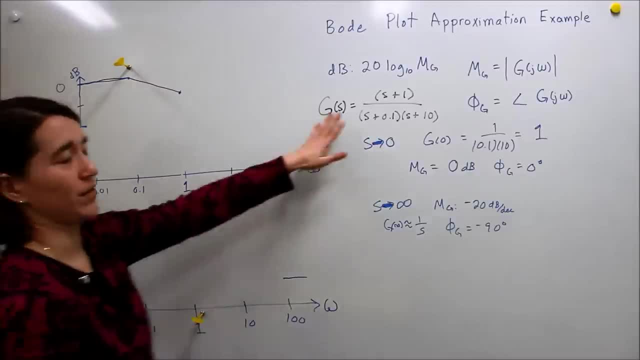 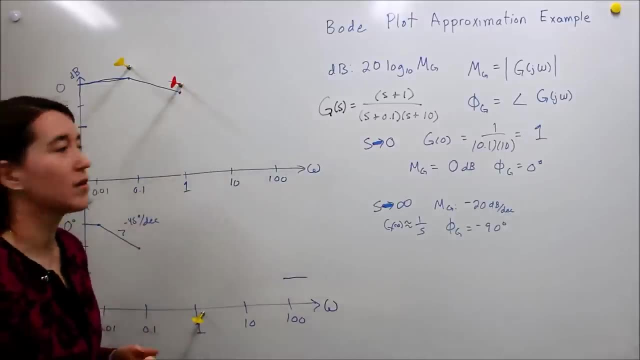 Okay, But now we have the effect of the next pole. Sorry, 0.. So the next one is 1.. So here we have 1. And in the magnitude we know it's going to do the opposite of the pole. 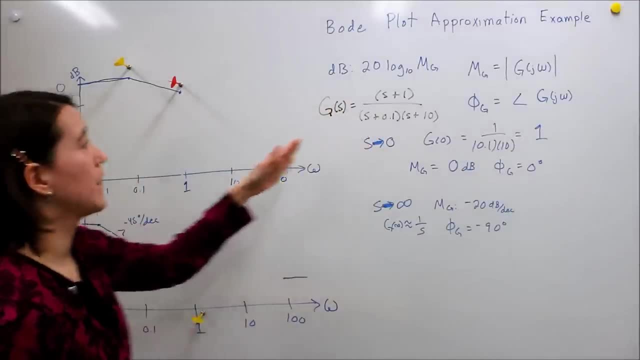 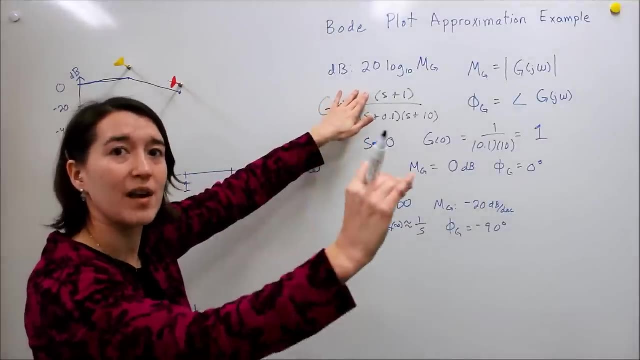 It's going to make the magnitude increase by 20 dB per decade. So we have the effect of this 0, which is making it decrease by 20.. This one is making it increase by 20.. So net we have 0.. 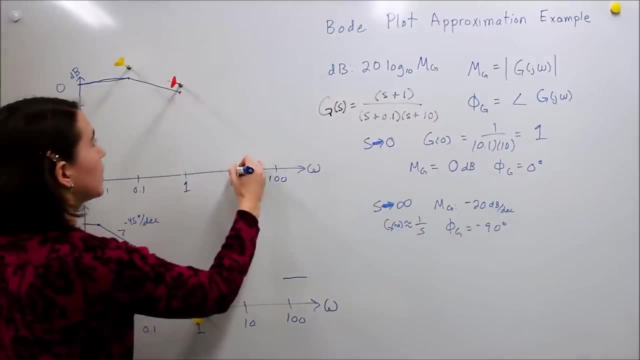 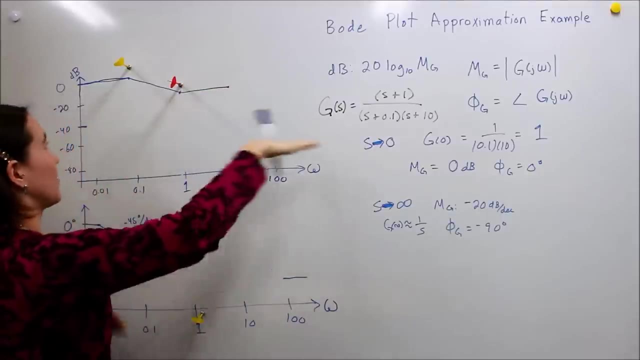 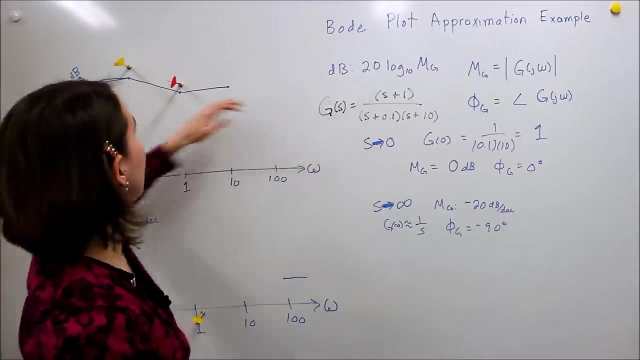 So what happens between here and our next pole- which we know is 10, is we're actually just going to see an approximate stability, So staying at one magnitude until we hit the next pole. So these two cancel each other out And that's what we're seeing in between these two points. 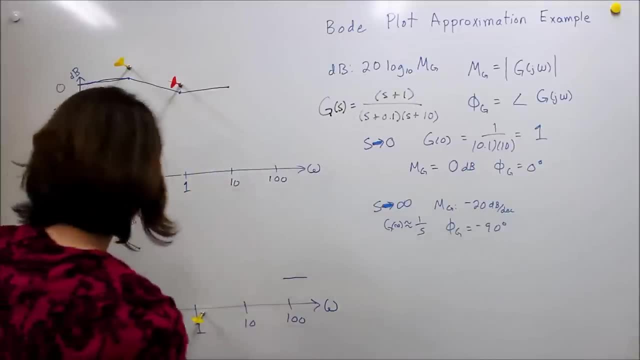 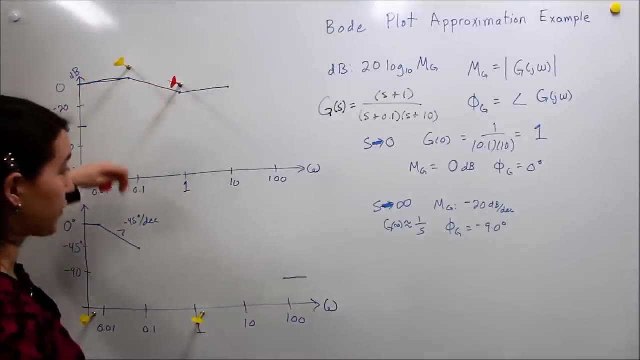 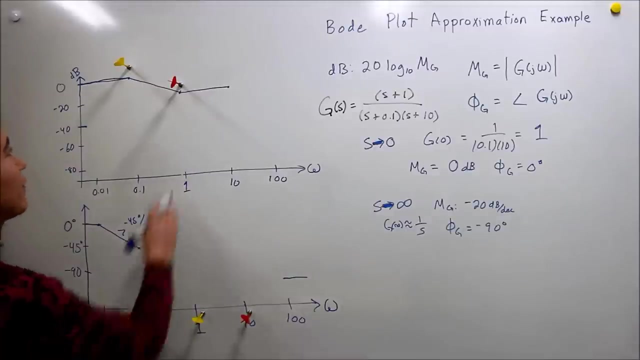 So between 1 and 10.. Okay, Let's look at the phase, how that affects the phase. So here again we have 1.. So the effect of this 0 will affect positive and negative 1 decade again. So once we hit this 0.1, we are getting the effect of this 0.. 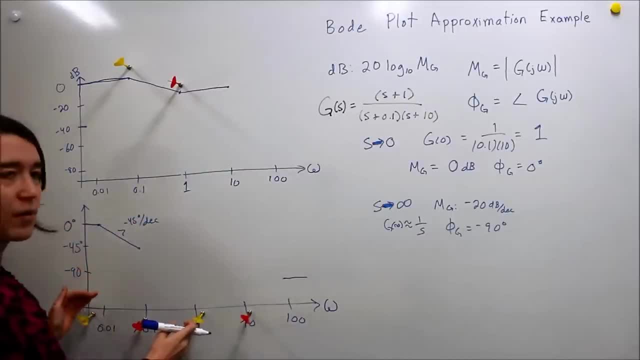 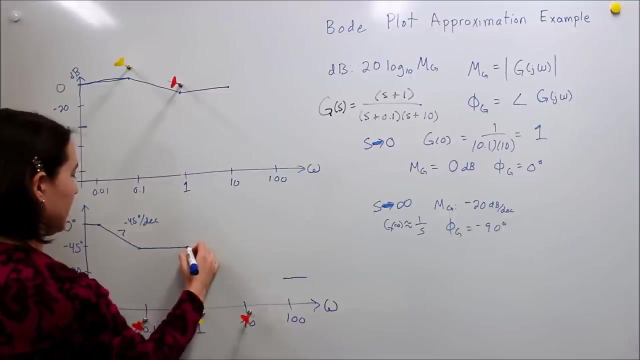 So between here and here we're decreasing by 45 degrees per decade, And between here we're increasing by 45 degrees per decade. So really we're again neutralizing. So we're actually just staying approximately at 45 until we hit the end of this effect. 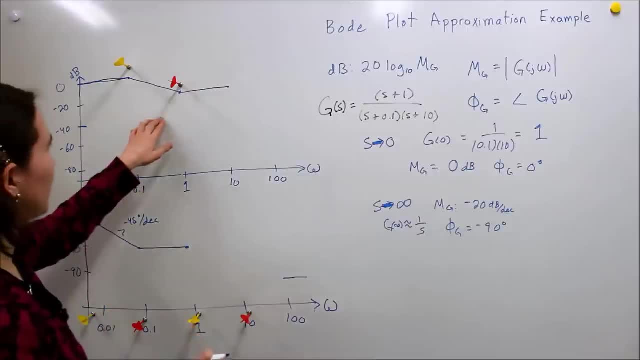 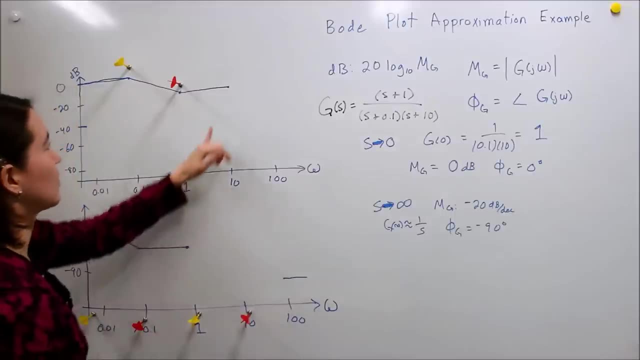 Okay, Okay. So if you're with me so far, it means we're looking good, Okay, So now we're going to move on to the last pole here, So that's at 10.. So we've hit this point. We don't have enough darts, so we have to reuse darts. 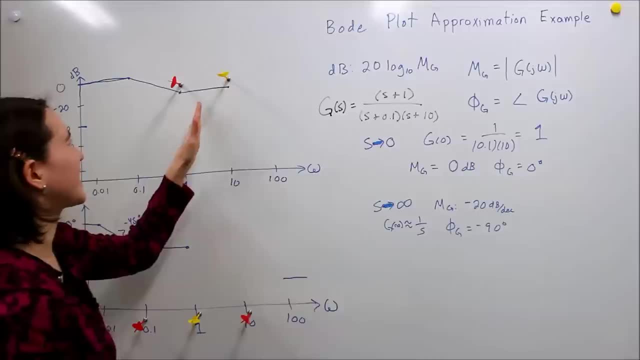 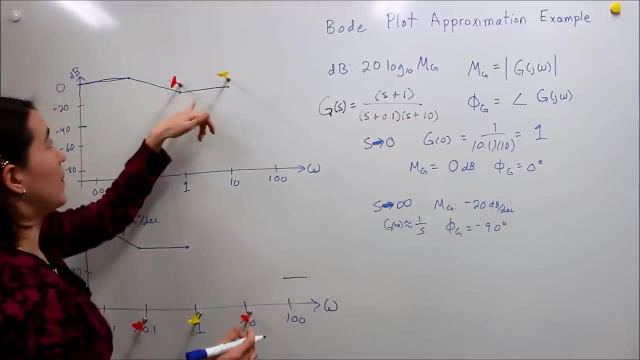 So here's our dart for the pole here, And now we're going to see the effect of this pole. Okay, So we're going to see the effect of this pole being added on to what was on here. So these two cancel each other out. 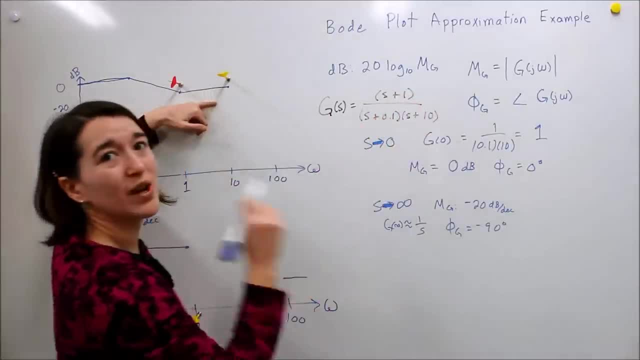 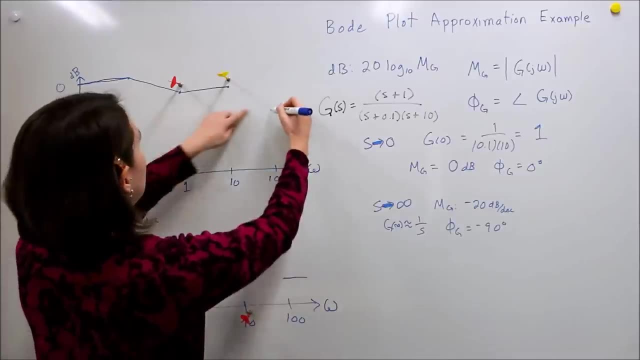 Negative: 20 dB per decade, positive: 20 dB per decade, And this last one is going to contribute another negative 20 dB per decade. So that's what we're going to see from this point on. So we're going to decrease here. 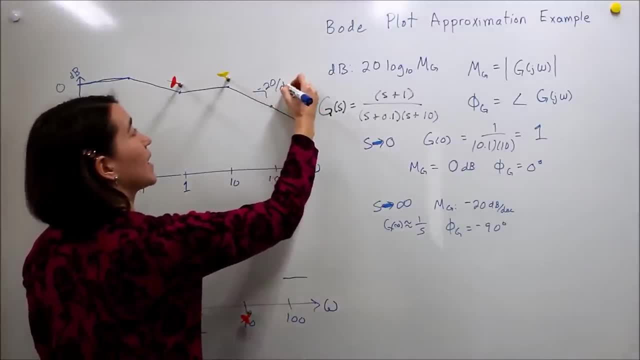 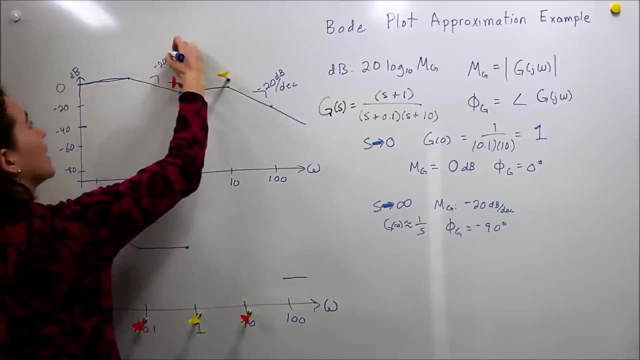 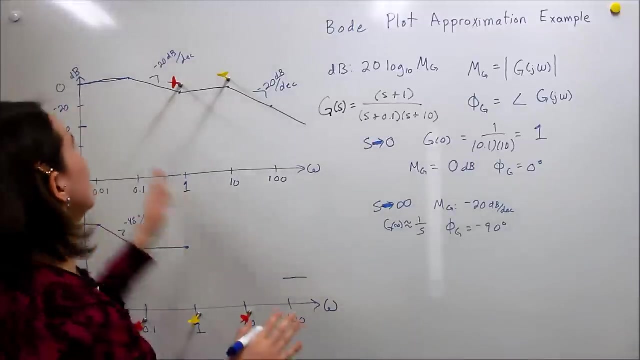 And we're going to just continue to decrease at 20,. negative: 20 dB per decade. dB per decade. Negative: 20 dB per decade. Okay, So this is the full magnitude plot, our approximation. So we see the effect of first the pole, then this zero and then this pole. 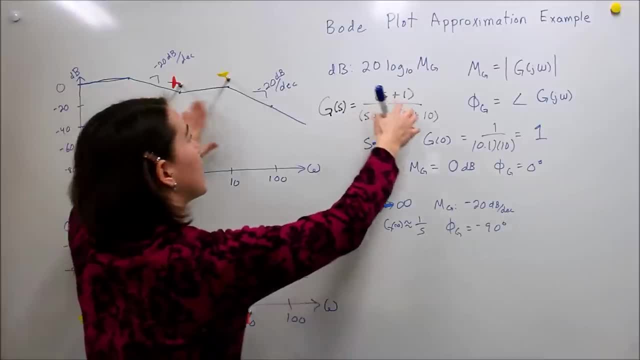 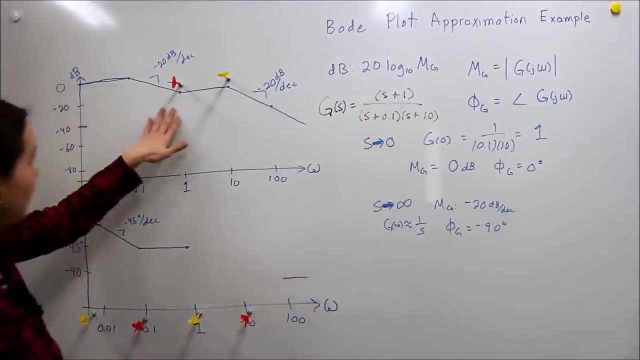 And then, as we go on to infinity, we just see the effect of this of one pole. Okay, So that's that. Now let's look at the phase one more time. So we've gotten up to this point on the phase. 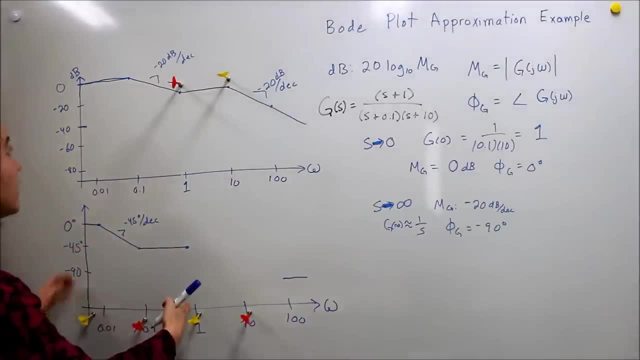 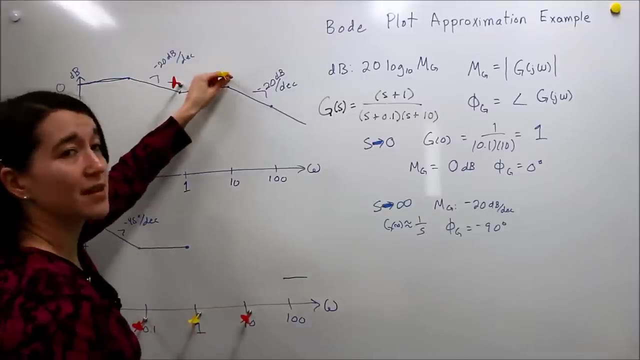 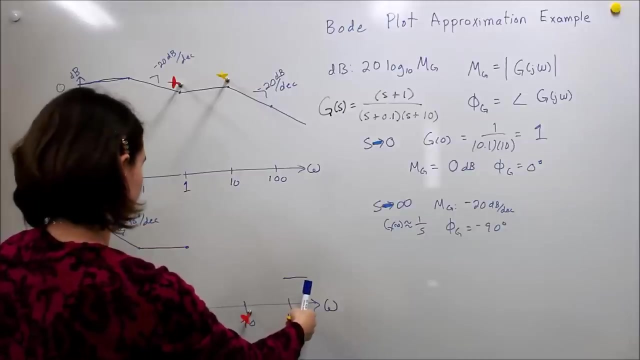 Now this pole is going to be negative 20 dB per decade. Okay, So now this pole no longer affects us after here, But we have the effect of this pole. So this pole turns out they overlap- affects one plus and minus one decade. 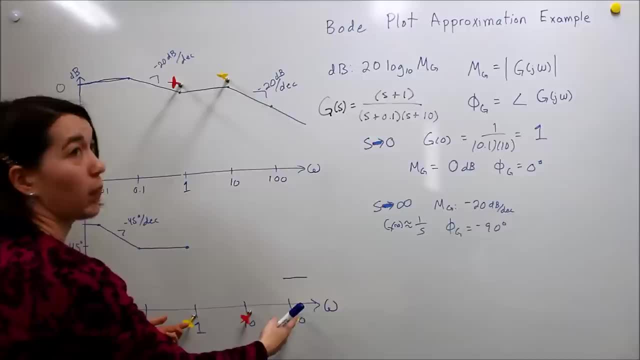 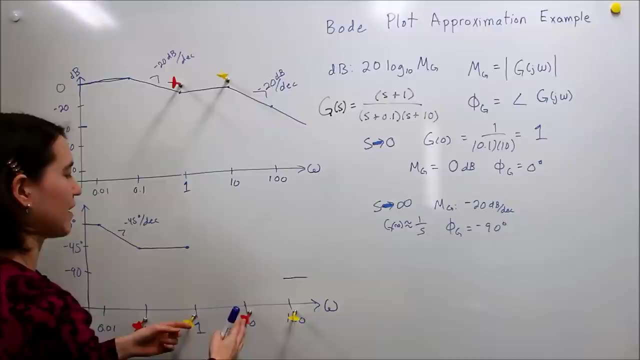 Right. So at one we're going to start seeing the effect of this pole. We already have the effect of this zero right. So here again, in between these two points we're actually going to, the two effects will cancel out. 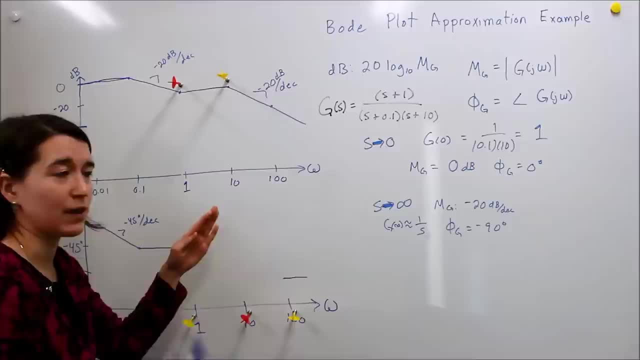 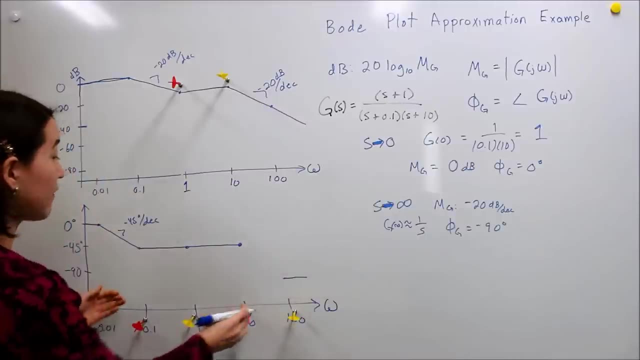 So one will want to increase by 45. By 45 per decade one will want to decrease Again. we get zero, So we get zero, up to this point, And then we reach the end of this: the influence of this pole. 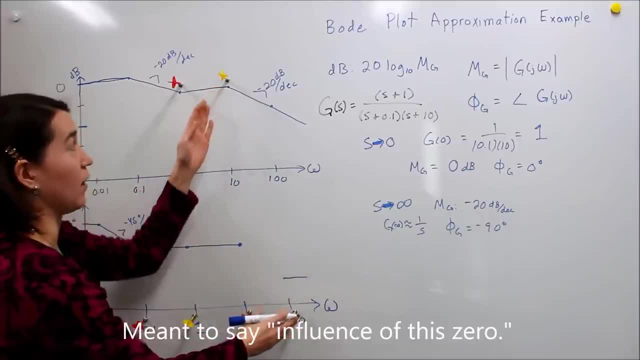 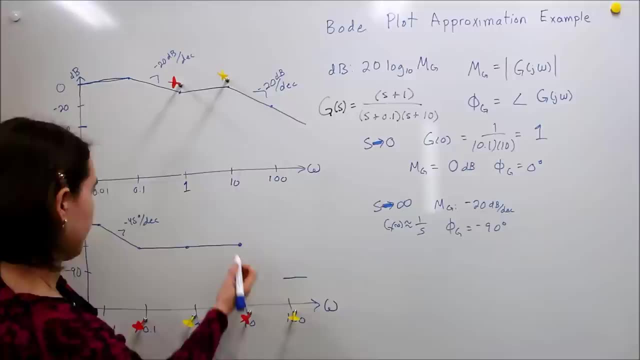 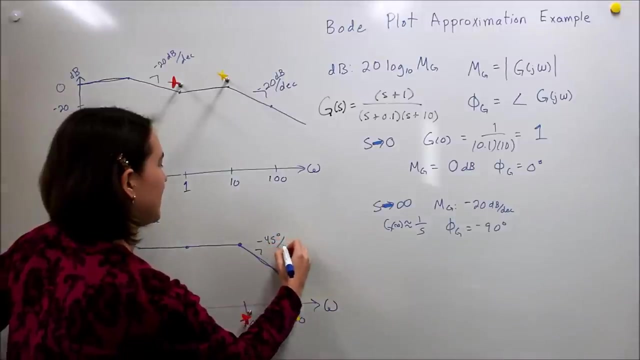 And now, between here and here, we just get the effect of this final pole at 10.. So we'll get a negative 45 degrees per decade. So here's that here, And I recommend labeling these, In case you're not as good of a drawer as I am. 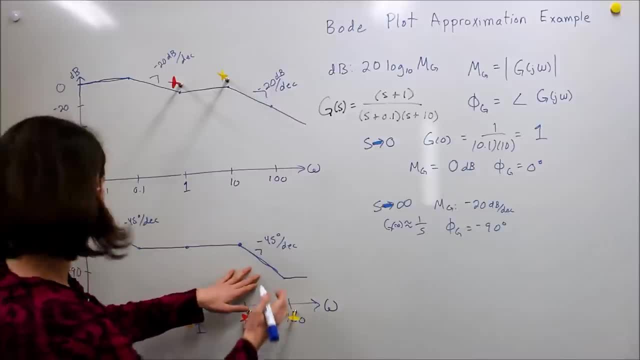 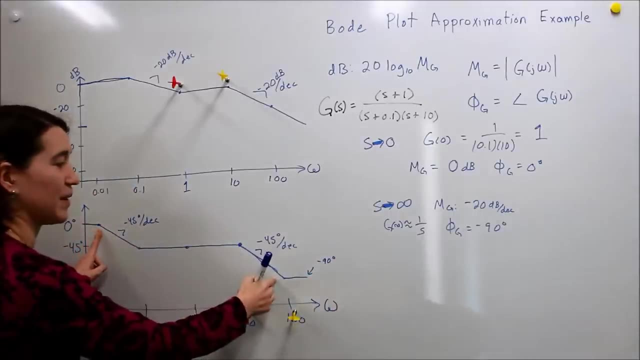 It's good to label them so that people know what the rate they are. And then this one we end at, just to clarify this- would be negative 90. So the addition of all these rates of angles should be the same, But we also already calculated that we need to end at 90.. 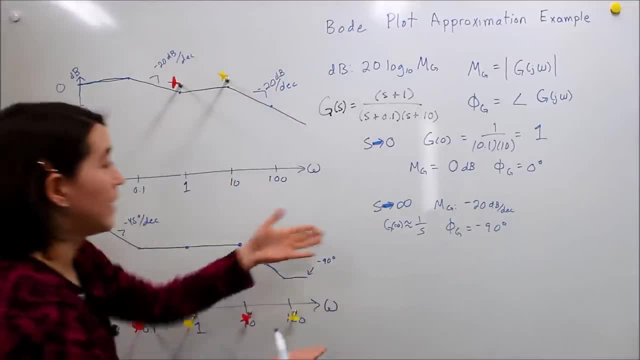 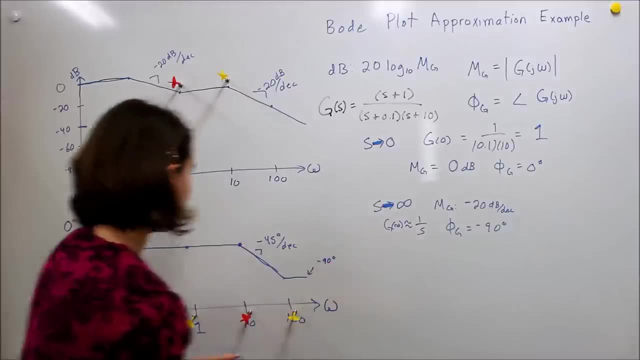 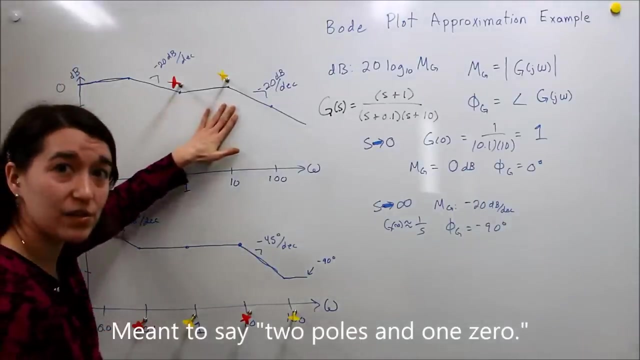 So we know our ending point here. Okay, And just to double check, we ended with a negative 20 dB per decade, which is what we expected as we go to infinity. Okay, We looked at the effects of each of the two zeros in the pole and the magnitude of our frequency response.